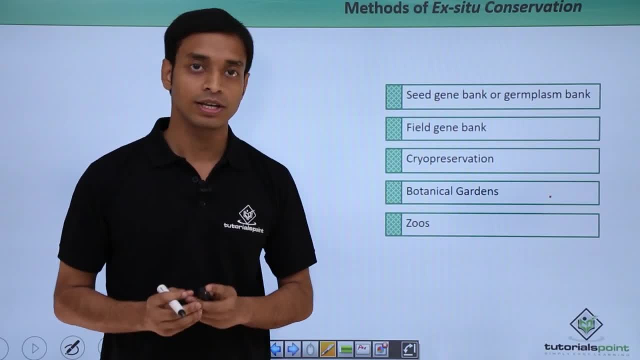 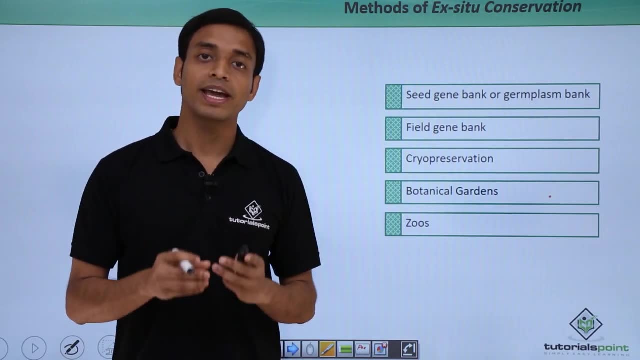 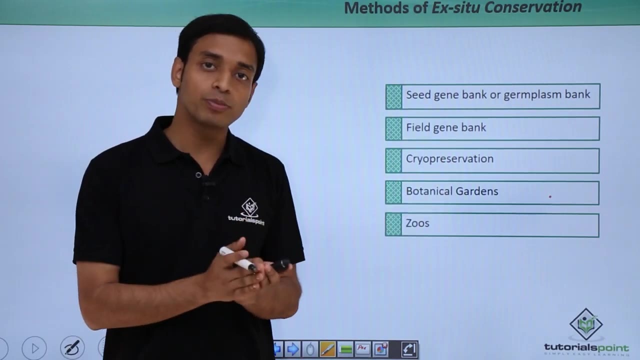 performed under specific controlled conditions. Now the next type or next method we are using is field gene bank. Here living samples of sperm egg embryo is conserved. The next type is cryopreservation, as we have already discussed, Like in cryopreservation, 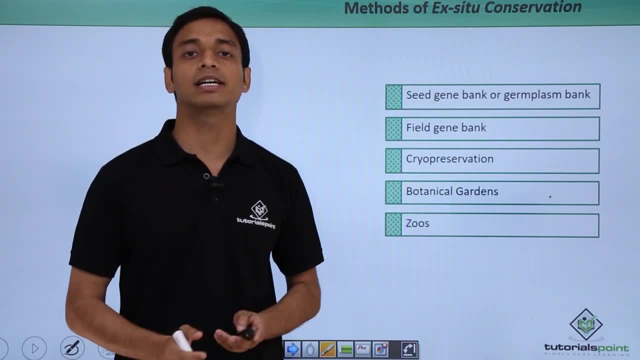 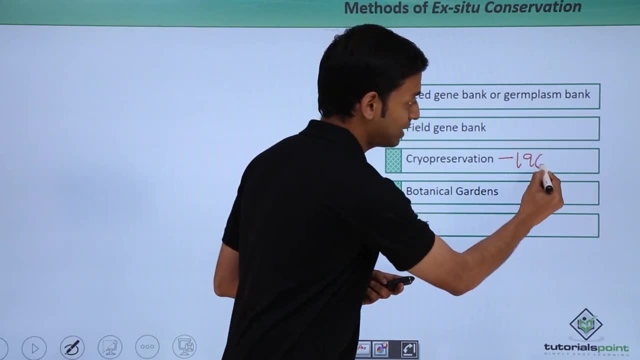 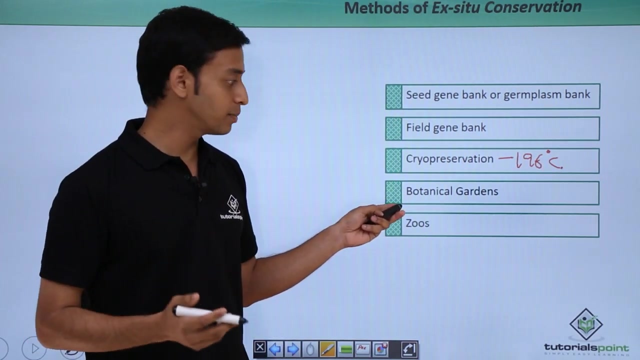 temperatures is very low and preservation is basically done at very low temperatures. The lowest we are talking about is the temperature of about minus 196 degree centigrade, and this is achieved by the use of liquid nitrogen. The next strategy is botanical gardens. You must be aware. 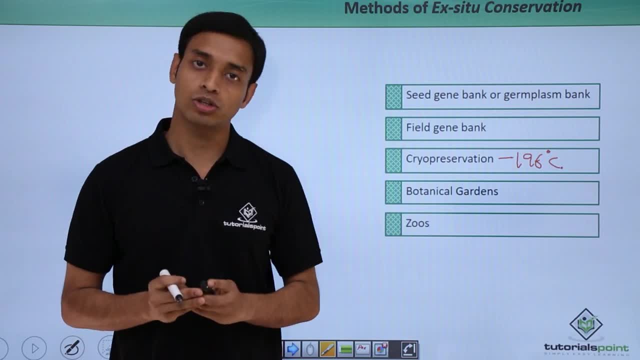 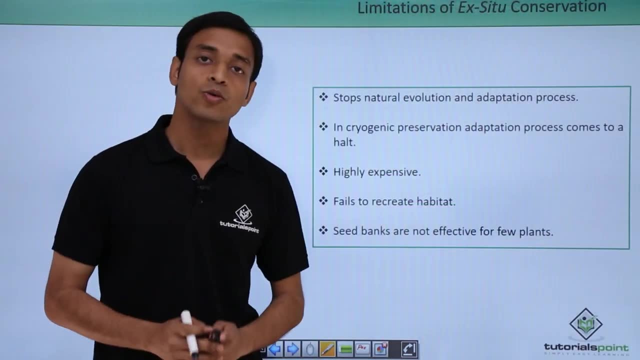 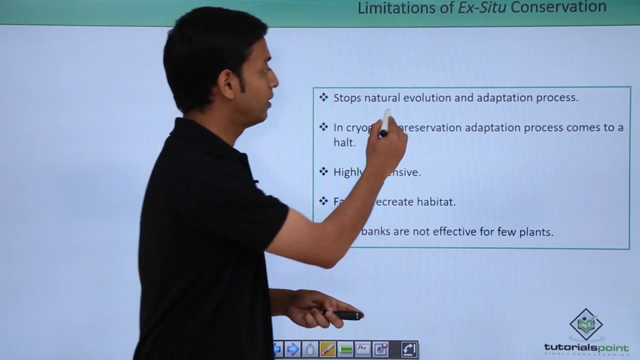 of this. These are areas where plant species are mostly protected, and the next is zoos or zoological garden, where animal species are protected. Now we are going to talk about some of the limitations of ex-situ conservation, The first one being it stops natural evolution and 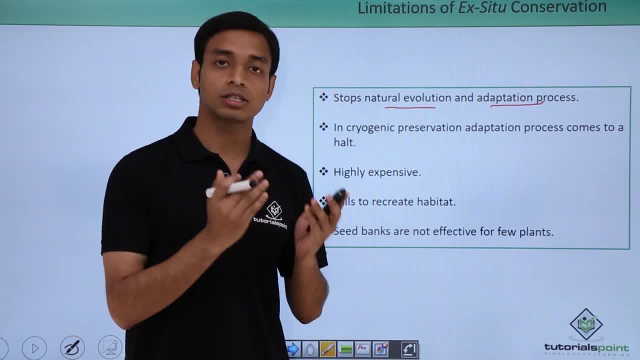 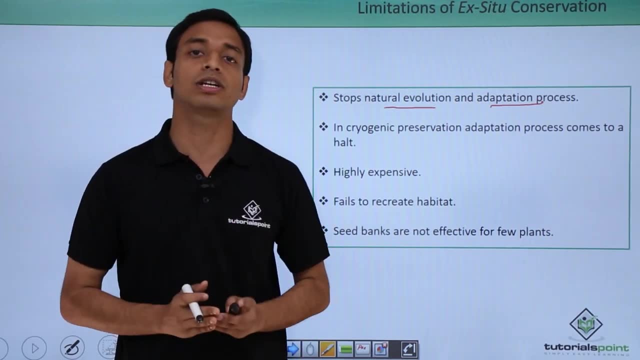 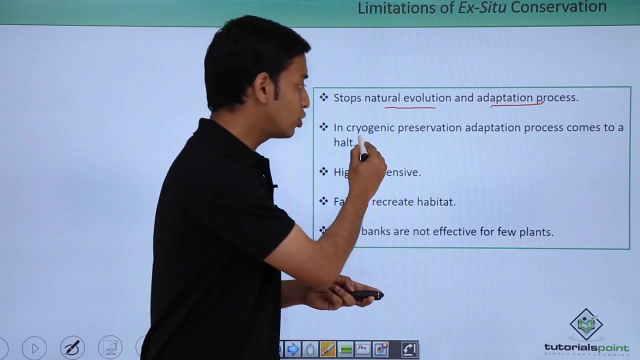 adaptation process because, you see, we are taking out the species of animals or plants from the natural environment and trying to preserve it in some artificial conditions. So the natural process of evolution and adaptation is coming to a halt Now because we are doing cryopreservation at very low temperature. the enzymatic activities and the metabolic activities. 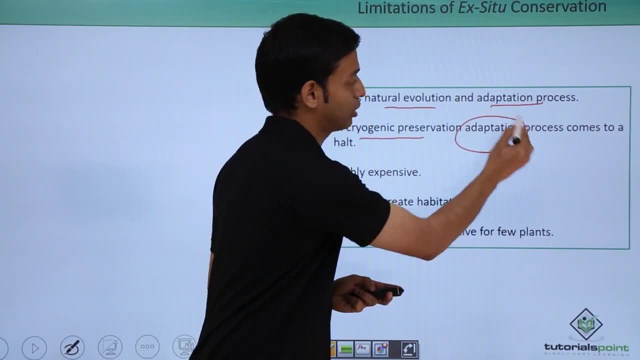 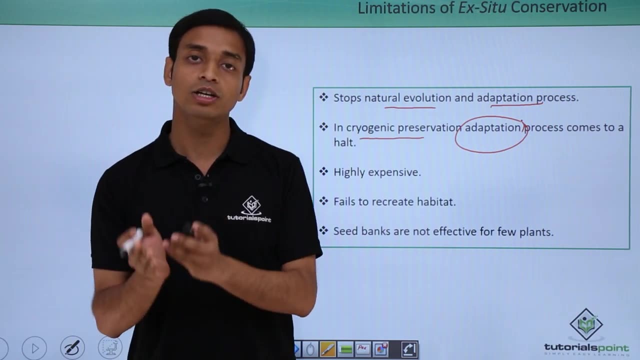 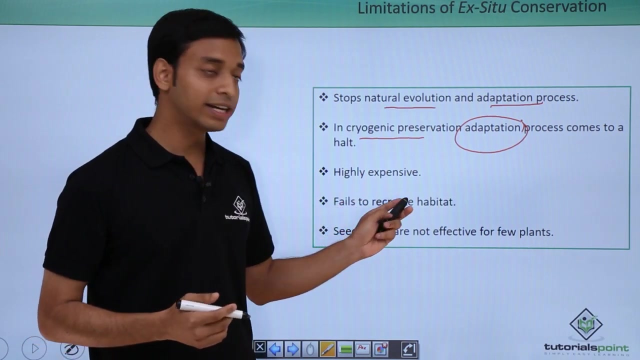 come to a halt. Hence the adaptation process is also stopping over here. Now, this is highly expensive because we are trying to create artificial environment which is similar to that of the natural environment, So it involves a large amount of money. The next is it fails to recreate. 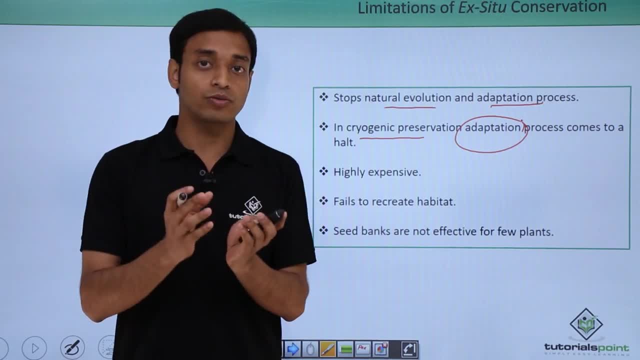 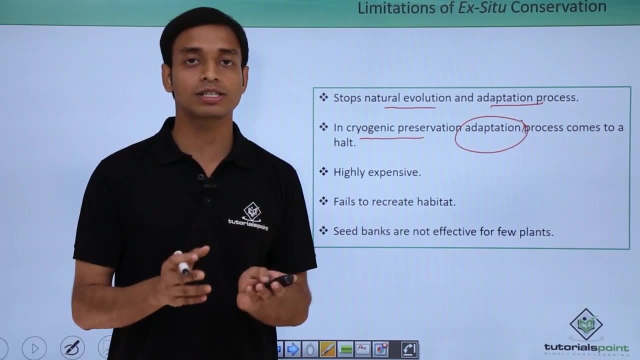 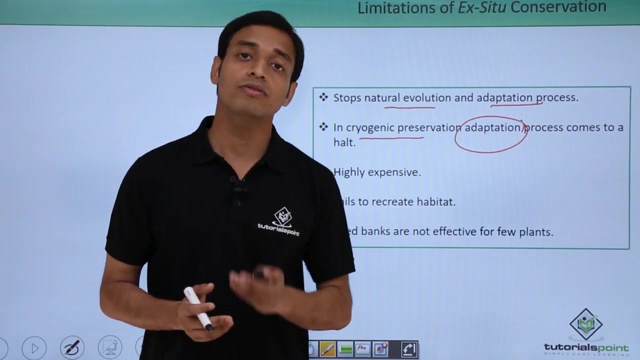 habitat. In this method we can use, we can. we are trying to conserve the species of plants, but we are unable to create the habitat as a whole because it's a artificial environment we are trying to create. And next is seed banks are not at all effective in terms of few plants, So in this video we have 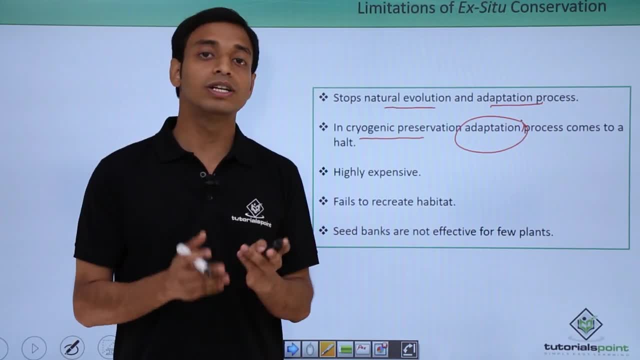 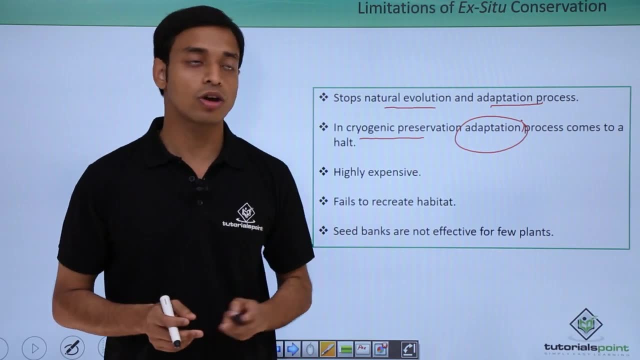 talked about ex-situ method of conservation. We have talked about the different methods or strategies we can use in case of ex-situ conservation. We have also discussed some of the methods we can use in case of ex-situ conservation. So I hope you have enjoyed this video. Thank you.